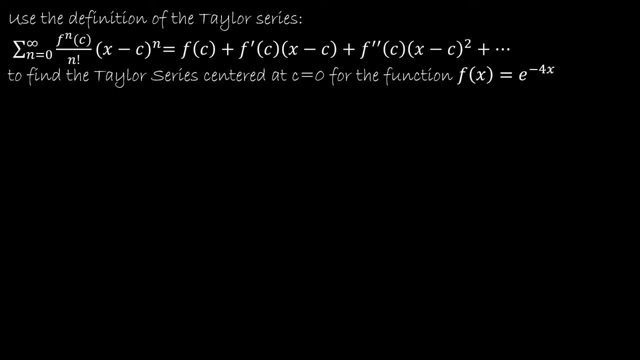 So let's do our first example together, and when we're dealing with the Taylor Series or McLaurin Series- which is technically what we have, when we have c is equal to zero- We're going to start by writing down the function, the first derivative of the function, the second derivative of the function, the third derivative of the function, and then evaluating each of those at the center. 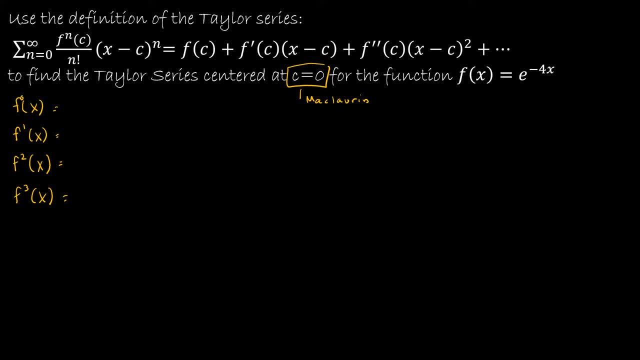 So this is technically like the zeroth derivative. So the first function is just what's given to us, which is e to the negative 4x. So that is not the derivative. That's the original function. The first derivative of the function is using the chain rule, which would be e to the negative 4x, then the derivative of negative 4x, which is negative 4.. 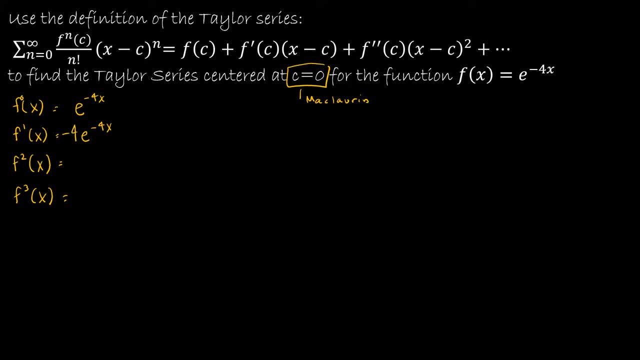 Continuing that strategy, I would take that expression times negative 4, which would make it positive 16 e to the negative 4x, and that expression times negative 4,, which gives me negative 64 e to the negative 4x. 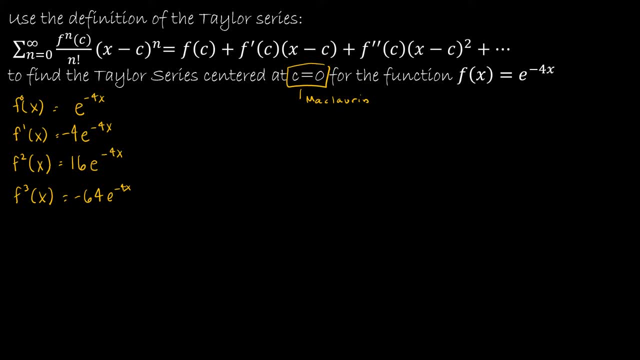 I'm then going to evaluate each of those at zeroth, Because that is the center. So now I'm going to find f of 0 at 0,, the first derivative at 0, the second derivative at 0, and the third derivative at 0. 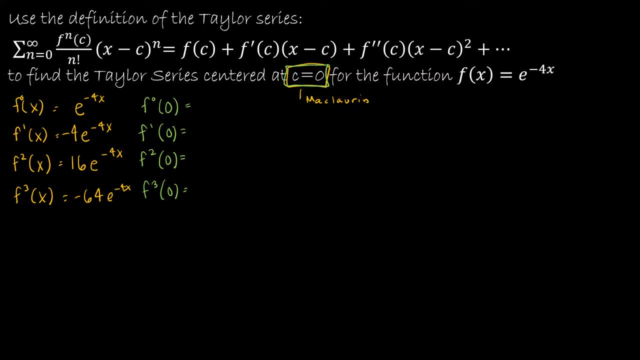 So that would give me e for my first one. This is obviously e to the negative, 4x 0,, which is e to the 0,, which is 1.. And then, using that same strategy, this is going to be 1,, but times negative 4.. 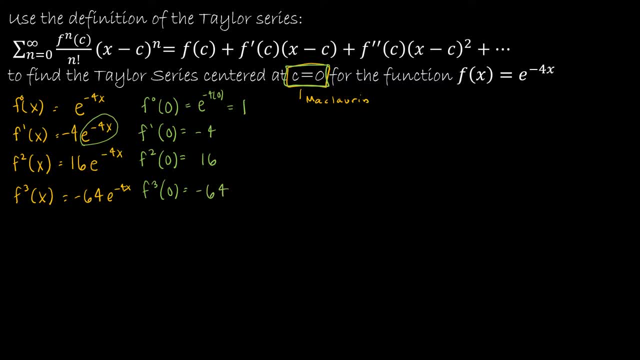 So this is negative 4,, this is 16,. this is negative 64.. Now what I'm going to do from here is start to write out my series. So e to the negative 4x. I can write it using this format. 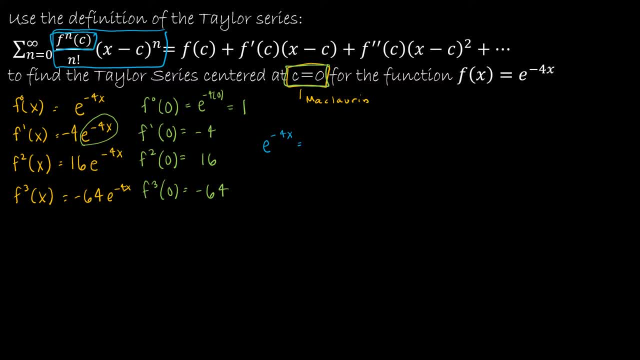 So this in the numerator is exactly what I've just found And that's why I wrote it in this way, with 1 and 2 and 3 instead of 1 dash and 2 dashes and 3 dashes. So my numerator for my first value, where n is equal to 0, would be 1 over 0 factorial. 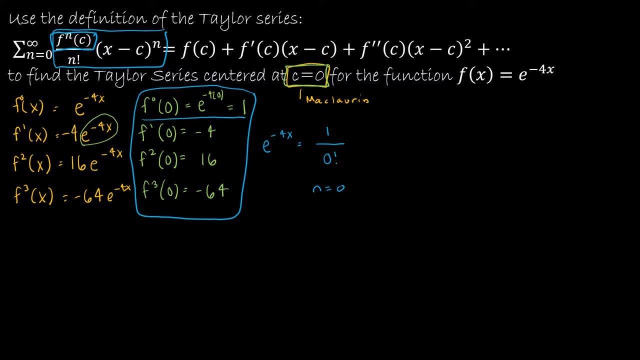 and then x minus c. now c is 0, so that's just x to the nth, power For n equal to 1, I'm going to, I'm going to now use negative 4, and then 1 factorial x to the first. 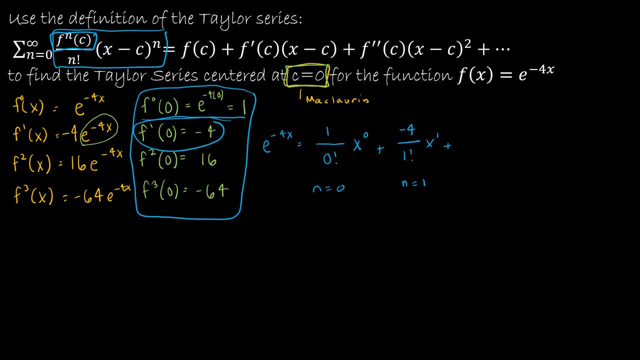 And then for f, the second derivative, it's 16, and then 2 factorial, because n is 2, x squared, and then negative 64,, 3 factorial, x cubed. Now what I'm trying to do is: 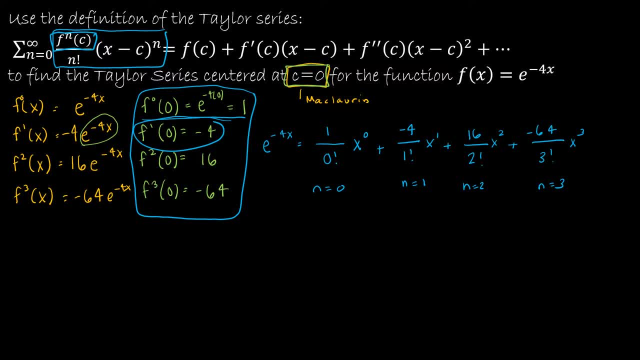 is. I want to write it as a summation, So I just want to simplify the pattern that I'm finding. So let's just do a little bit of simplification. e to the negative 4x. My first value is 1 over 0. factorial x to the 0.. 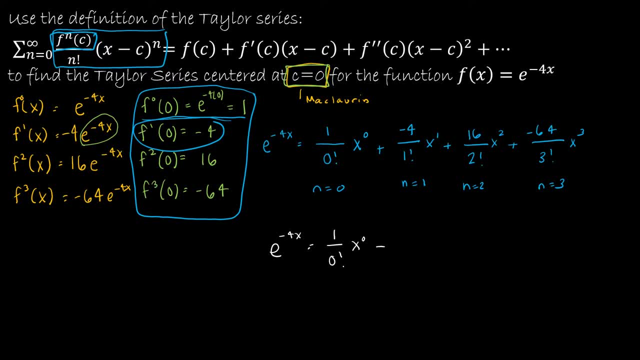 My second value is now minus 4 over 1.. 1 factorial x. my third value is 16,, which I'm going to write as 4 squared over 2 factorial x squared, and my third value is negative 64,. so I'm subtracting. 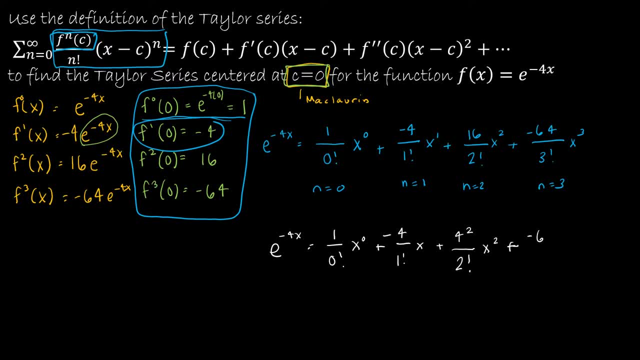 actually let's go ahead and leave the negatives on there. So plus negative 64, and 64 is 4 to the third. So 3 factorial x cubed, and of course this continues forever. Now, why did I want to write it in that way? 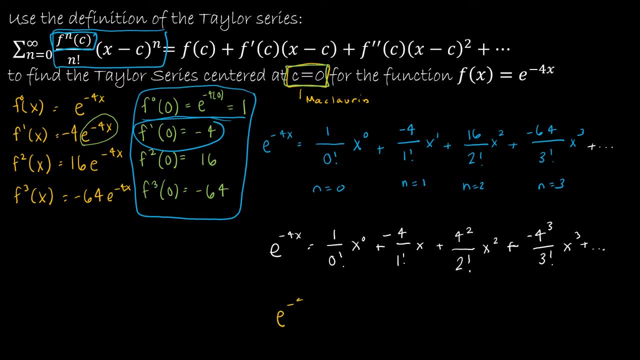 Because I want to be able to write this as an infinite series. So the summation is oops, as n goes from 0 to infinity of what. So let's just take a look at what's happening. This value is positive. 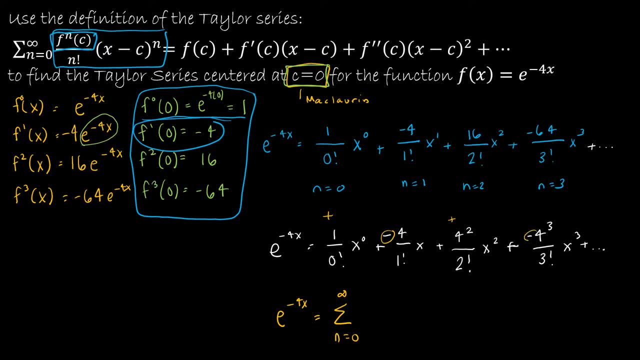 This value is negative, This value is positive, This value is negative, And so I know that's just an alternating series. So it's either going to be negative 1 to the n or negative 1 to the n plus 1.. 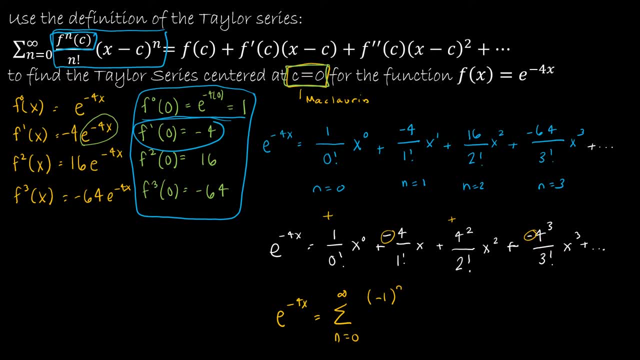 Since my first value is positive, it's negative 1 to the n. That makes all of the even values positive. Then what do I have? I have 4 to the first, x to the first, 4, squared, x squared. 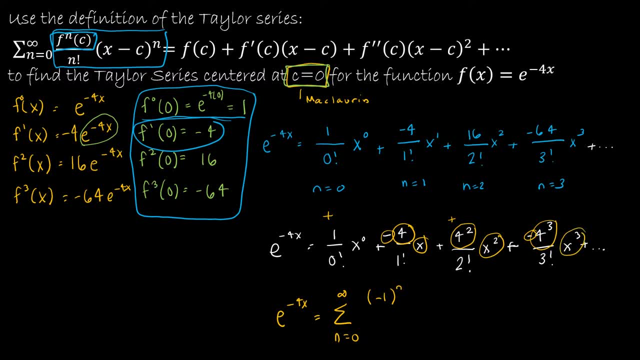 4 to the third, x to the third. So that means I'm going to write 4x to the nth, Because, remember, this was n1,, n2, n3, and so forth. And then in my denominator I have 1 factorial, 2 factorial, 3 factorial. 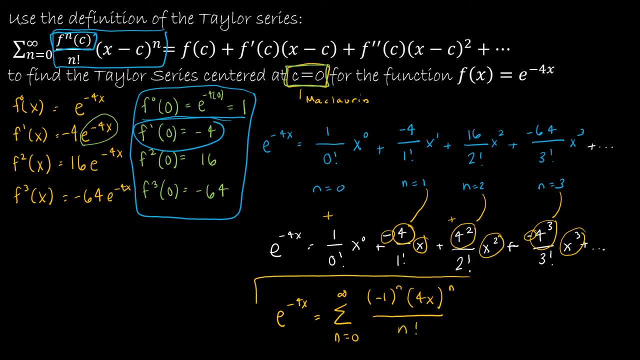 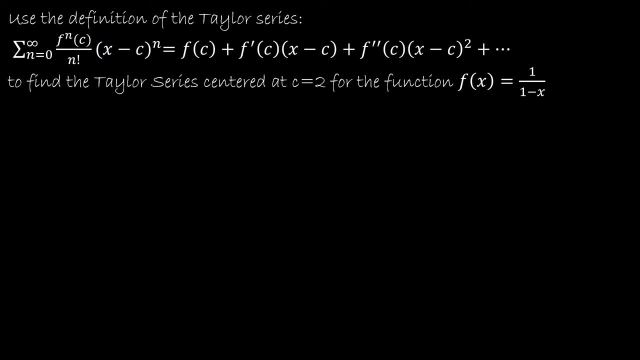 So that's just n factorial. So I have now successfully written e to the negative 4x as a power series or a Taylor series. All right, let's try another example using the Taylor series. Again, this one is not going to be centered at 0, so it is a true Taylor series. 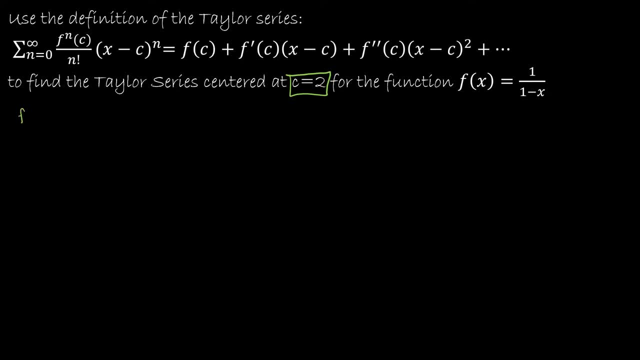 But we're going to go about this in the same way we did before. I'm going to use my original function, which is 1 over 1 minus x, And again, if they didn't specifically ask me to use the Taylor series, I would probably not. 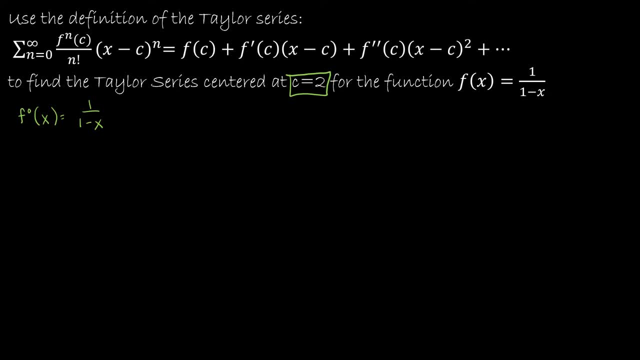 I would probably use the strategy we learned previously using the geometric series, because this would work very well. So I'm going to use the geometric series, But we'll go ahead and use this because they've asked us to. I'm going to rewrite that function as 1 minus x, to the negative first. 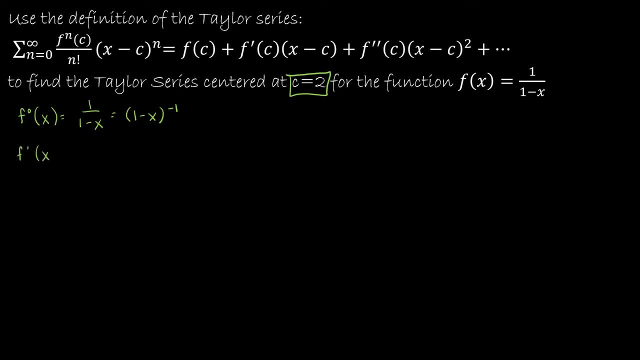 So the derivative function. the first derivative would be, using the power rule, negative 1, 1 minus x to the negative 2.. And then the derivative. I'm sorry, the chain rule says: now take the derivative of 1 minus x. 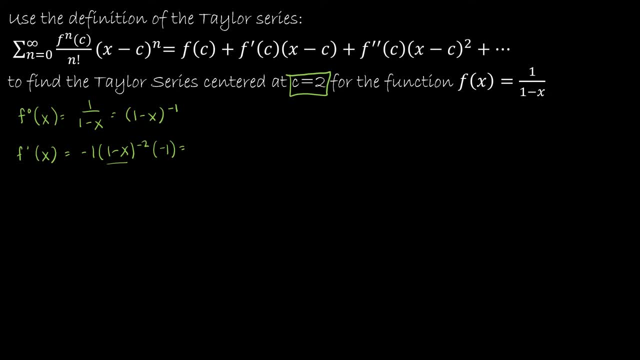 which is negative 1. So that turns into positive 1.. 1 minus x to the negative: 2. Then the second derivative using that same strategy would be negative 2, 1 minus x to the negative, 3 times negative 1,. 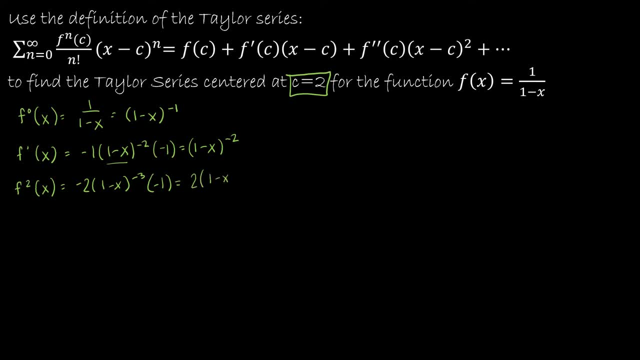 or positive 2, and then 1 minus x to the negative 3.. And then the third derivative would again be using negative 6, 1 minus x to the negative 4th times negative 1, or positive 6,, 1 minus x to the negative 4th. 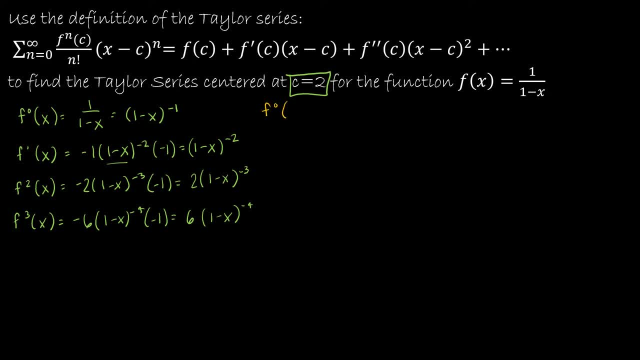 Now, if I'm going to find each of those values at 2,, for the first value would be 1 minus 2, so negative 1 to the negative 1st, or 1 over negative 1 to the 1st, which is negative 1.. 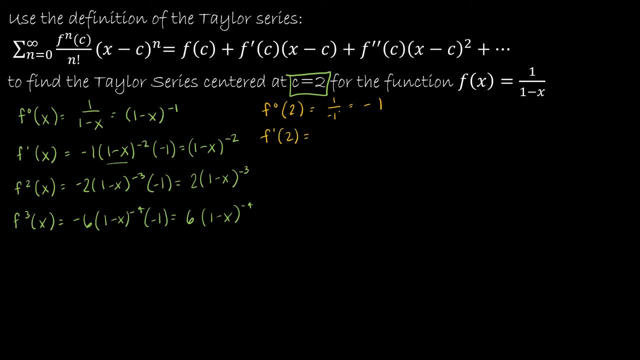 The first derivative at 2 would be 1 over negative 1 squared, which would be 1 over positive 1, or 1.. The second derivative at 2 would be 2 over negative 1 to the 3rd, which is 2 divided by negative 1, or negative 2.. 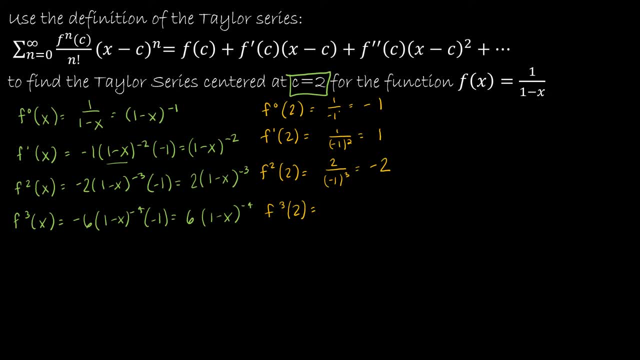 And the third derivative at 2 would be positive 6 over negative 1 to the 4th, which gives me positive 6.. Now let's use all of those values. So we're going to use all of those values to rewrite 1 over 1 minus x, using our definition. 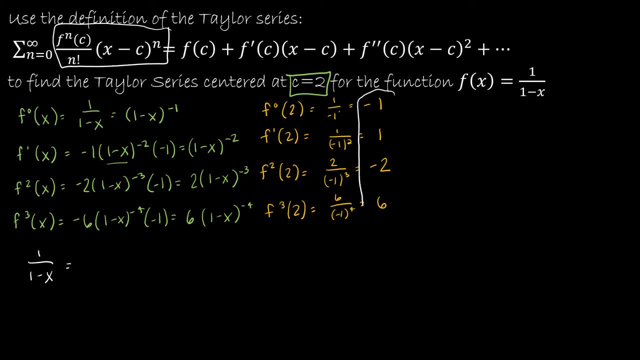 So I'm going to start with these coefficients, that's my numerators. that's why I had to find them over n factorial, and then x minus c to the nth. So the first guy is negative, 1 over 0 factorial. 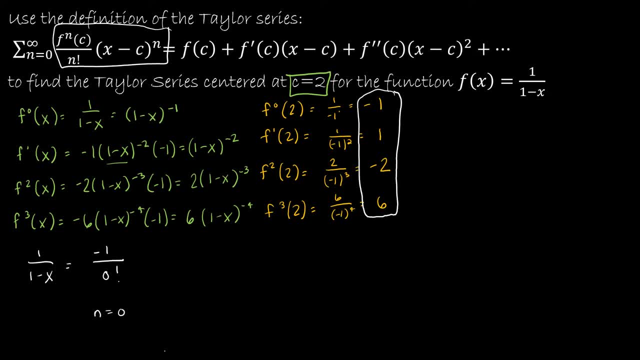 because the first guy is: when n is 0, of x minus c, so x minus 2, of x minus c, so x minus 2, of x minus c, so x minus 2, to the nth power and n is 0. 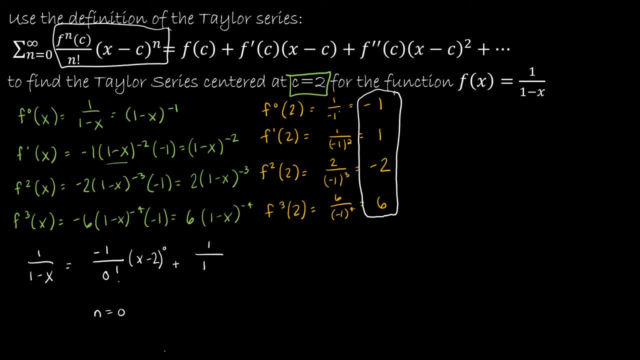 And then the next one is 1 over 1 factorial, because n is 1, and then x minus 2 to the 1st, and then I have negative 2 over 2 factorial, and this is x minus 2 to the 2nd. 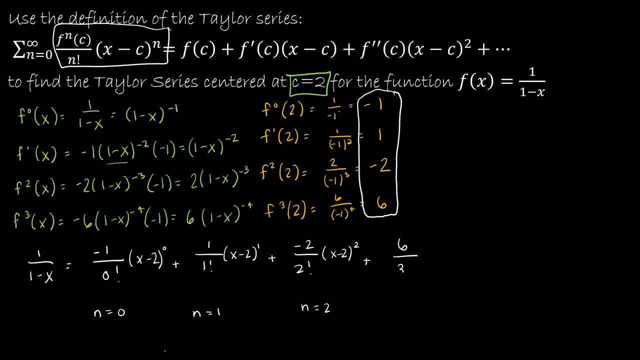 and then I have positive 6, over 3 factorial, and then x minus 2 to the 3rd, and this pattern would continue. So I'm gonna get these out of the way, just because I don't have room for that. 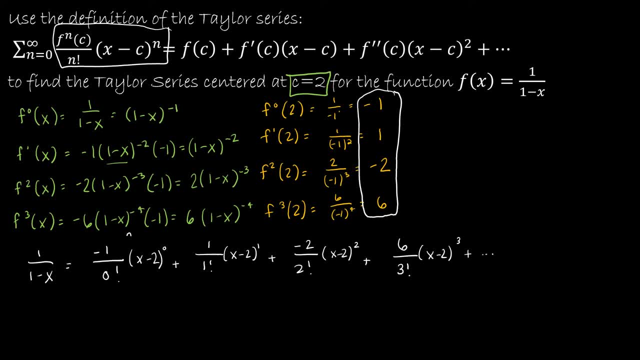 But keep in mind that that's what we're doing- is: n is 0,, n is 1,, n is 2, n is 3, and the pattern continues. So I just need to think about how could I rewrite this. 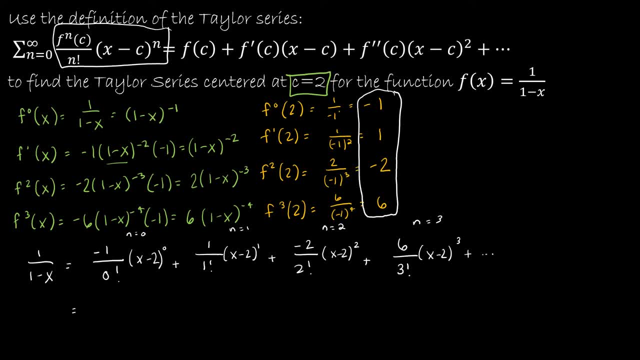 How, what do these values work for me? So I just need to think about how could I rewrite this? how, what do these values work for me? equal. so sometimes it's better to go ahead and evaluate this. so the first guy is negative 1 over 0 factorial, which is 1. so this guy is negative 1, and then X. 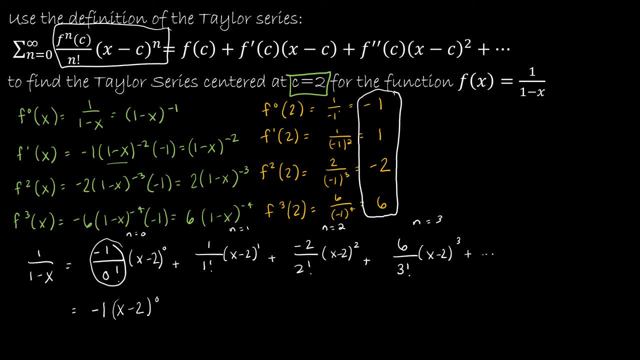 minus 2 to the 0, and this one is positive 1. 1 over 1 factorial, which is 1, and then X minus 2 to the first, and this is negative. 2 over 2 factorial is 2 times 1, which is 2, so negative 2 over 2, which is negative 1, and then X minus 2. 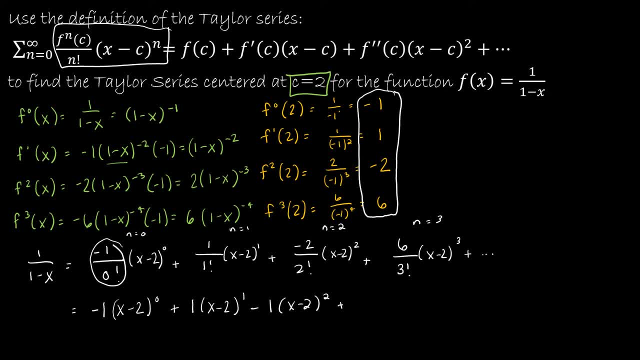 squared. and then the next one is 3 factorial 3 times 2 times 1, which is 6. so that's 6 over 6, or one X minus 2 to the 3rd. so I can see. the pattern now is that the coefficient is negative. 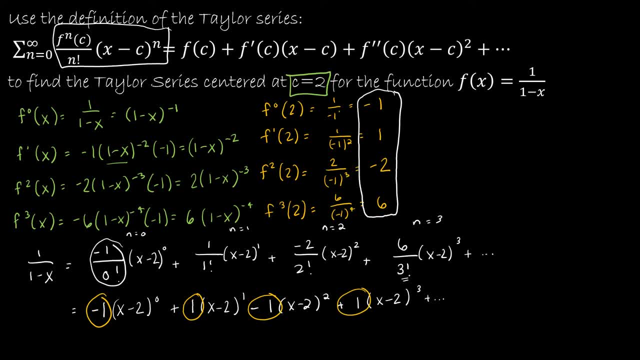 negative 1 to the 0. this is a failure. so we have to be aware that there are and positive 1 alternating And so, because my first guy is negative, I can write 1 over 1 minus x as negative 1 to the. I'm sorry, I need to write the summation first. I'm getting ahead of myself. 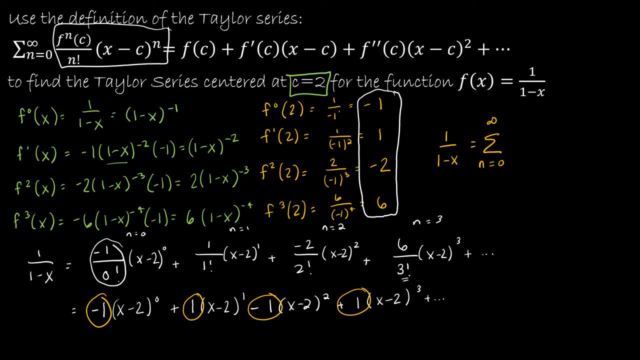 This summation as n goes from 0 to infinity, of negative 1 to the, not n, because if I used n then the first value would end up being positive. So this is n plus 1 times x minus 2 to the n, And that should give me the correct value. And again, you can always. 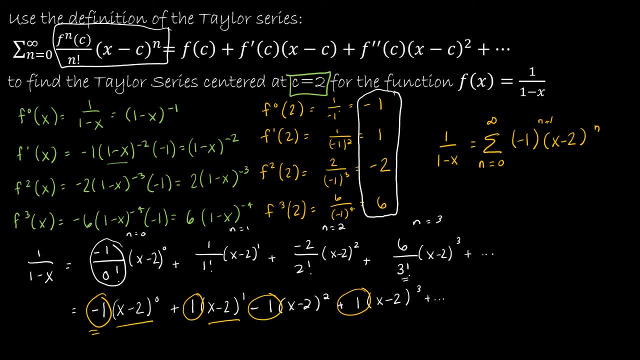 just do a test to see if it works. So, especially if you're dealing with the negative 1 and making sure that you have the correct sign, If I plugged in 0, that would give me negative 1 to the 0 plus 1, which is to the first, and then x minus 2 to the 0. Does that give me the correct? 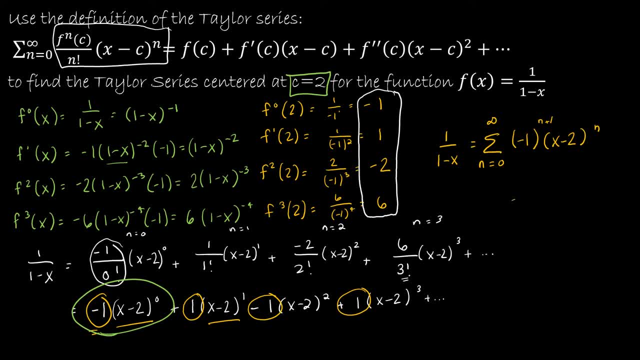 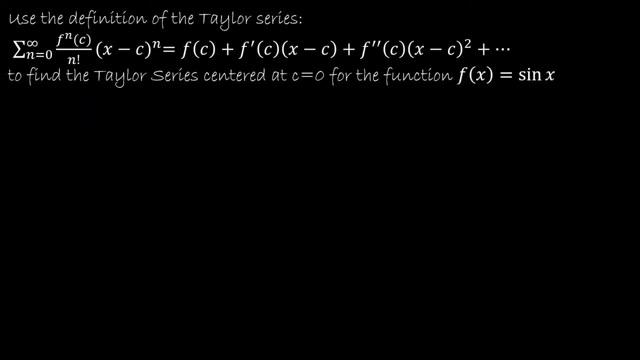 value here? Yes, it does. So I'm convinced, And we'll just go with that. Here is my final solution. Let's do just one more example, And in this example I want to use a trigonometric function, because we haven't dealt with those in a while, And you should always be dealing with trigonometric. 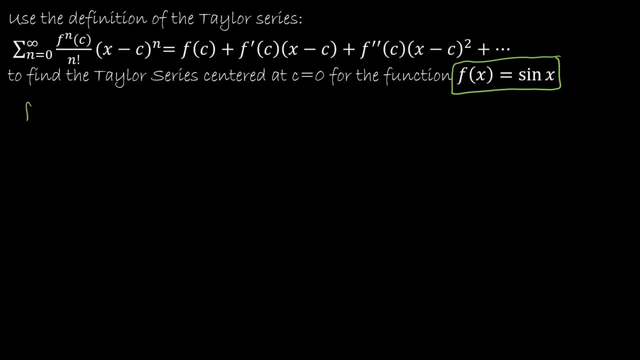 functions. So we'll start with the original function. We're going to start with the original function, The original function which is, of course, sine of x. The first derivative, which is cosine of x, Derivative of sine, is cosine. The second derivative, which is negative, sine of x. 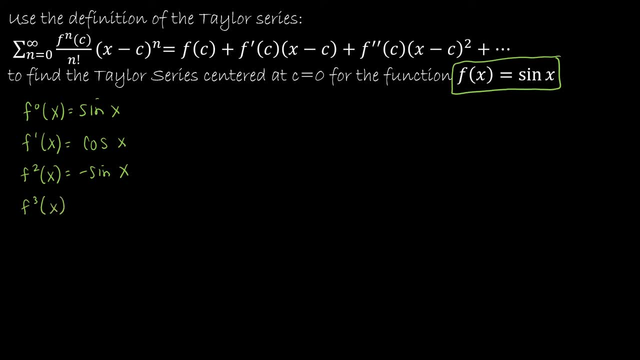 The third derivative, which is still using that negative, So negative cosine of x. And then the fourth derivative would be the derivative of cosine of x, Cosine which is negative sine, but now it's negative negative sine, so it's positive sine. 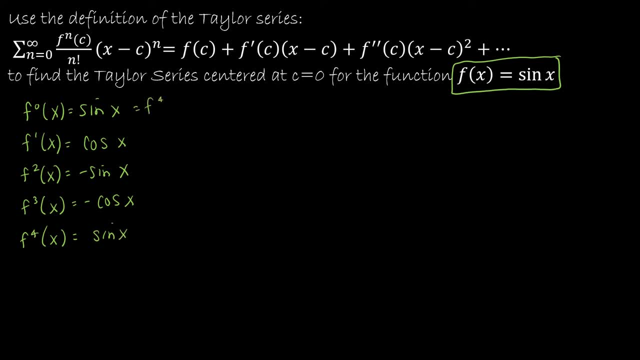 So, as I can see, this guy would be the fourth derivative and the fifth derivative and the sixth derivative, and so on. So this is f6 and f7, and continuing forever. So now let's evaluate those functions at zero. If I take the function of sine of zero, I'm going to get zero. 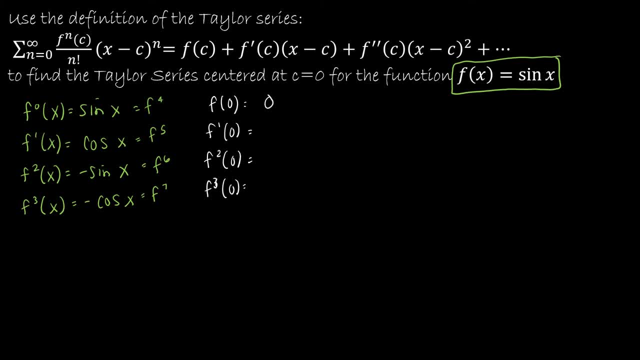 And if I take cosine of zero, I'm going to get one, And negative sine of zero, I get zero. And negative sine of zero, I get negative one. And that pattern would continue and continue, and continue and continue. So, just as we have in our last examples, I can say: f of x or sine of x is equal to zero. 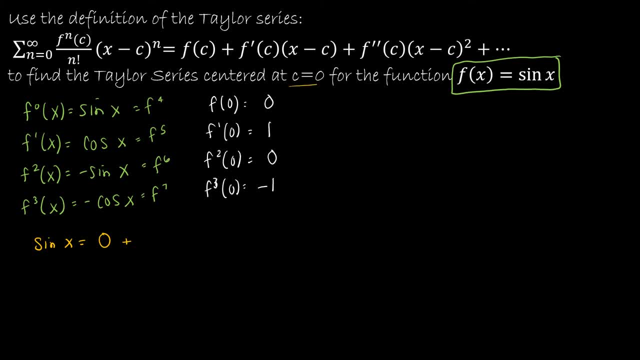 And then again c is zero. So it would be zero over zero factorial and then x to the zero, And then I would have one over one, One factorial x to the first and zero over two factorial x squared and negative one over three factorial x cubed. 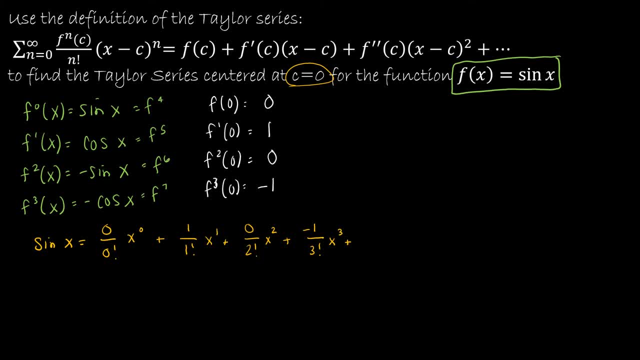 And then the coefficients would continue to alternate: zero for factorial x to the fourth, positive one x factorial- I'm sorry- five. factorial X to the fifth, zero, six. factorial x to the sixth, negative one, seven. factorial x to the seventh, and so on. 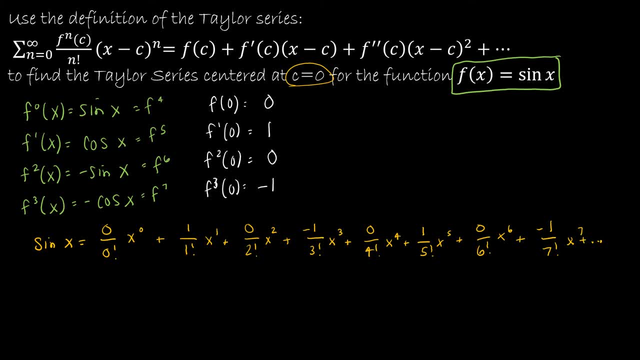 And you might be thinking: well, geez, we don't usually do that many terms, But the reason I did so many is because this guy is obviously a zero, and this is a zero, and this is a zero and this is a zero. 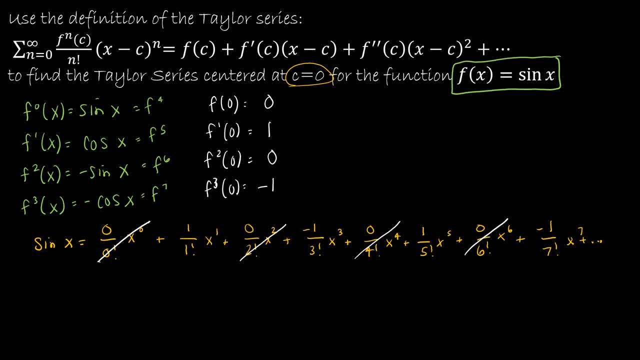 So every other term is canceling out. So I now have sine of x. It's equal to one over one factorial, which is just one x to the first. So my first one is one x. My next term is negative: one over three factorial. 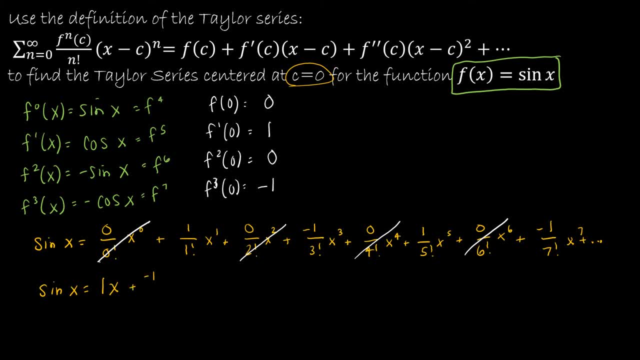 So it's negative one x to the third over three factorial, And then positive one x to the fifth over five factorial And negative one x to the seventh over seven factorial, and so on. That's why I did so many, because all of those zeros canceled out and I needed enough left over to come up with a pattern. 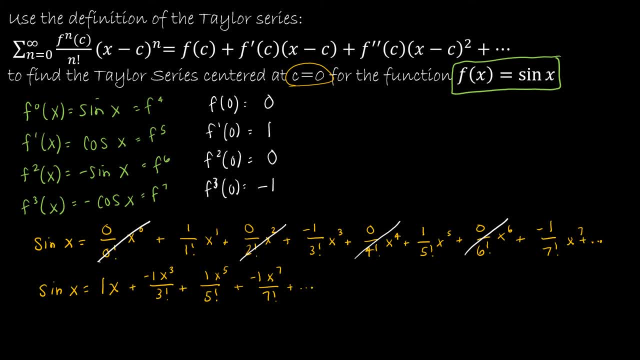 So now, what I need to think about is the fact that this is when n is zero and this is when, I'm sorry, this is when n is one, And this is when n is three, And this is when n is five And this is when n is. 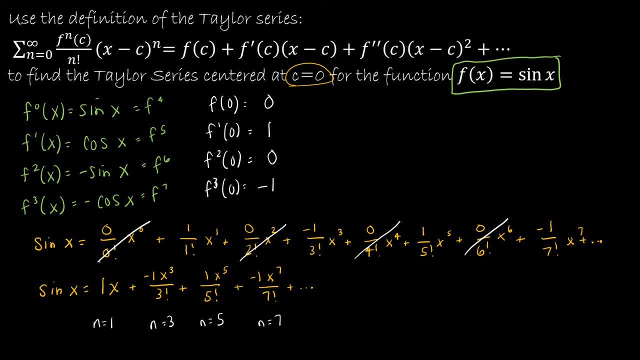 Seven, And so I need the even ones to essentially go away And I need the odd value. So I need really. what I want to do is rewrite my function. So let's do sine of x. I want to rewrite it so that when n is zero, I get this value. 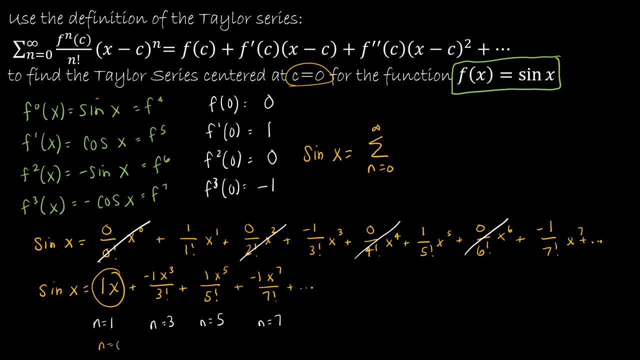 And when n is one, I get this value. So how am I going to make this work? I really just want the odd values. So I'm going to essentially look at the fact that one and one factorial three factorial five, factorial seven factorial- this is just an arithmetic sequence. an arithmetic sequence has the first value of one and it goes up by the common difference. so that's one plus two n. 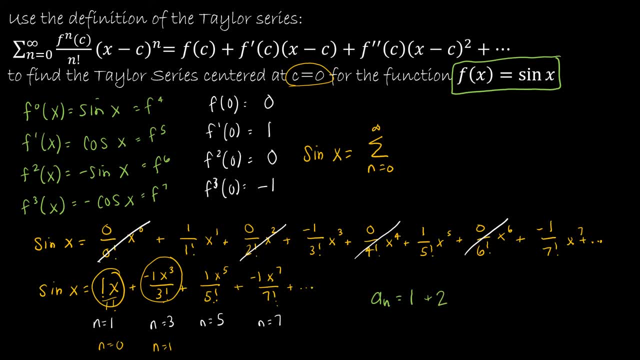 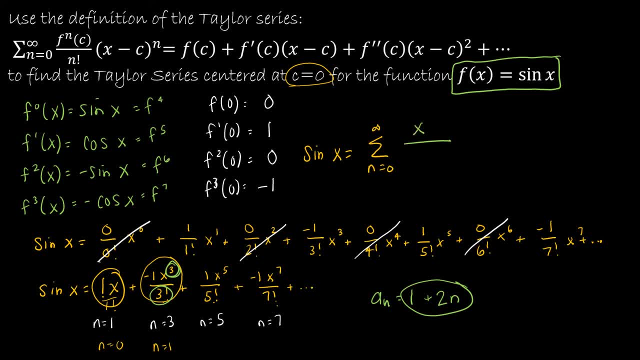 So I get x to the two n plus one, which is the same as one plus two n divided by two n plus one factorial. So let's talk about the negative part in just a moment. So let's talk about the negative part in just a moment. 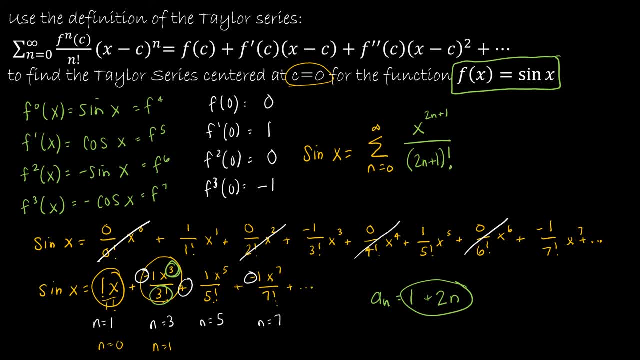 Because obviously this is an alternating sequence- negative, positive. But so far let's see if I'm on the right track. If I chose, n is zero, that would give me x to the two times zero plus one. so x to the first and then two times zero plus one, one factorial. 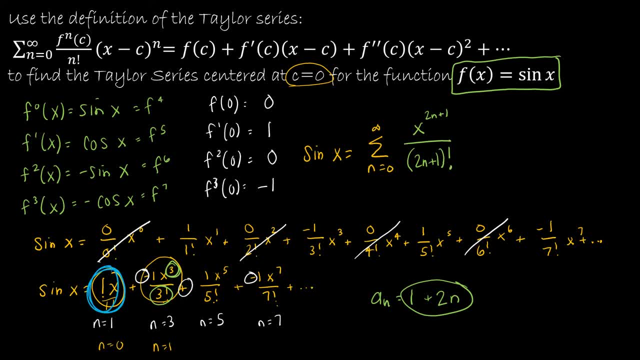 That gives me my first value. Let's look at my second value. My second value should be negative and we'll deal with the negative in a minute. So that means, if I plug in one x to the two times one plus one is three over two times one plus one is three factorial.